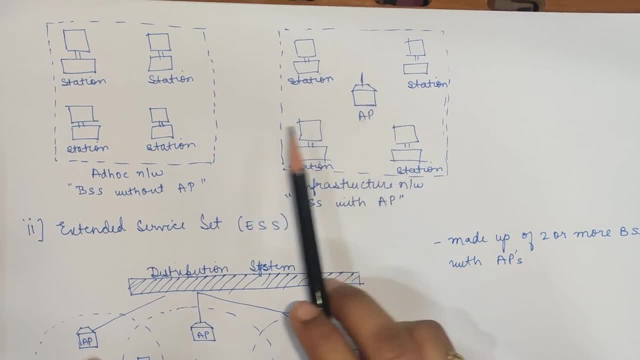 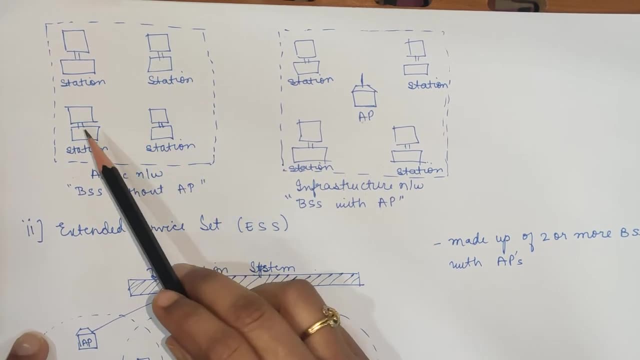 So if it can directly communicate in this station, what is in this BSS? what is going to happen? they can directly communicate, But what happens If one station want to communicate with another BSS station? they cannot communicate because it does not have an AP. 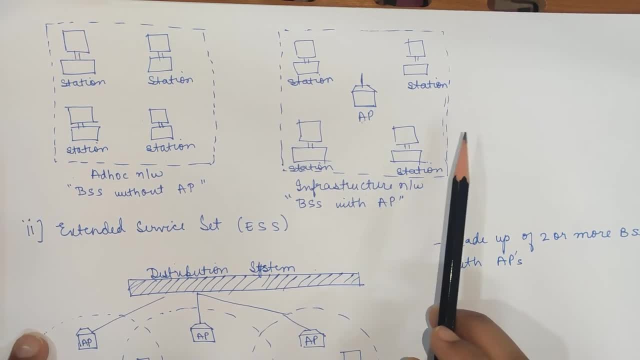 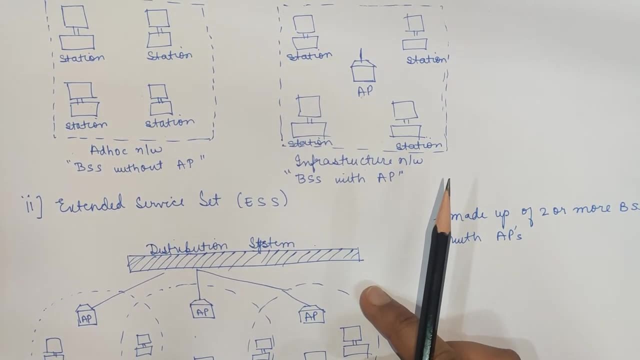 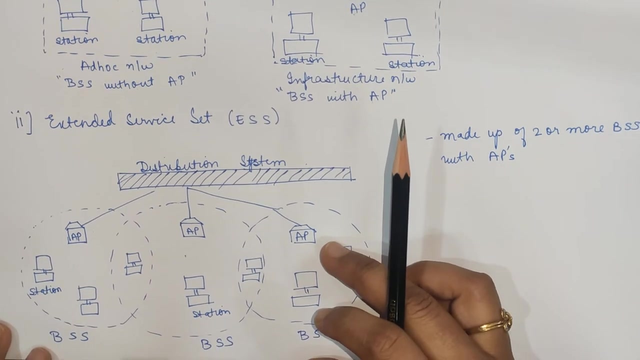 Whereas in this case they can communicate with the other BSS stations. See what is happening: if you want to communicate with another stations of another BSS, we have to use an extended service set service. So what is happening in this we will see. See extended service set. it is made up of: 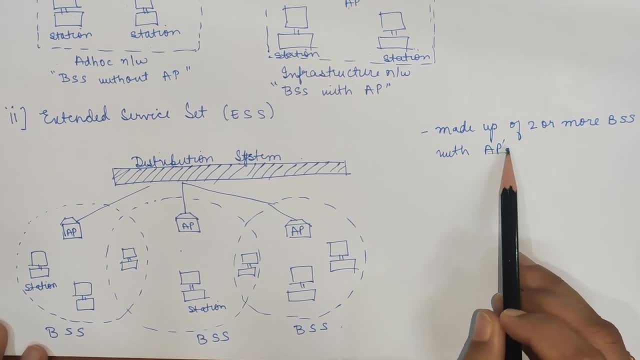 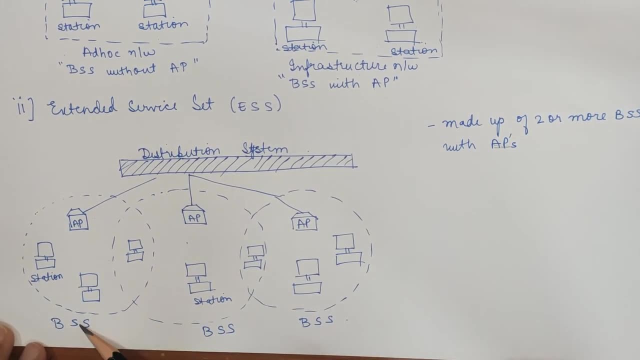 Two or more BSS with an access point made up of two or more BSS. as you can see in this diagram, there are three different BSS, or you can say basic service set. all are having an AP and that all are connected to a distribution system. 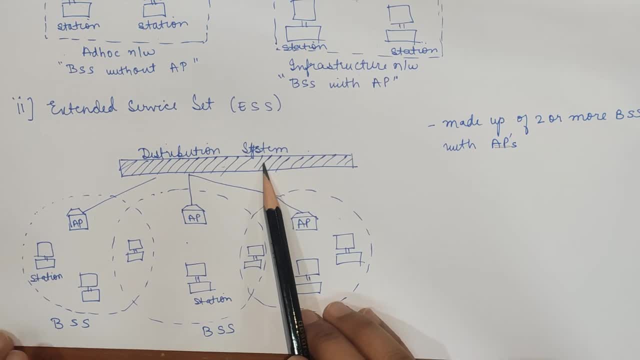 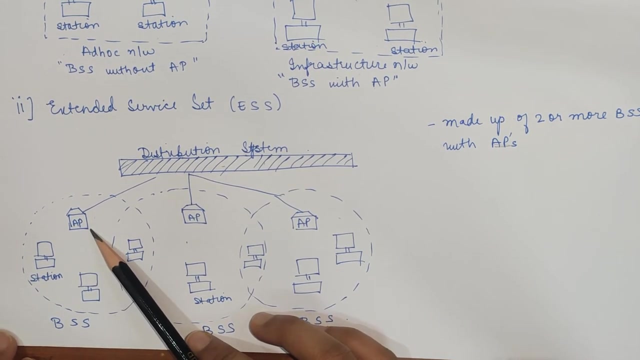 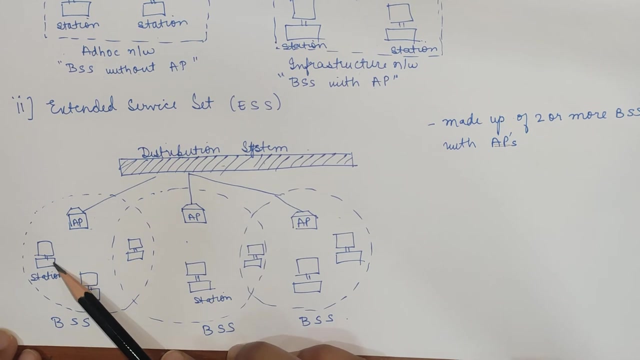 All the access points are connected to a distribution system, See communication between two stations of one BSS. Two stations of one BSS can communicate directly. can communicate directly through an AP, Okay, but what is happening here? you should know. if we want to communicate with like, for example, if station, or if we want to communicate if this station wants to communicate with this station and this of these are obviously of different BSS. 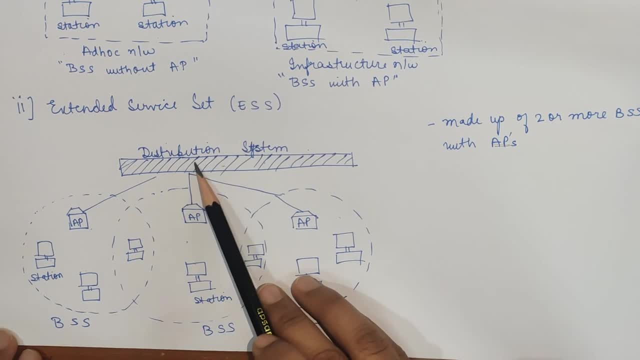 They can communicate via a access point, but it is obviously going to communicate via distribution System, means stations sends the respective message or a frame to the access point and that is obviously connected to the distribution system and then it is conveyed to. the message is conveyed to the respective access point and then again the message is going to convey to the destination address. 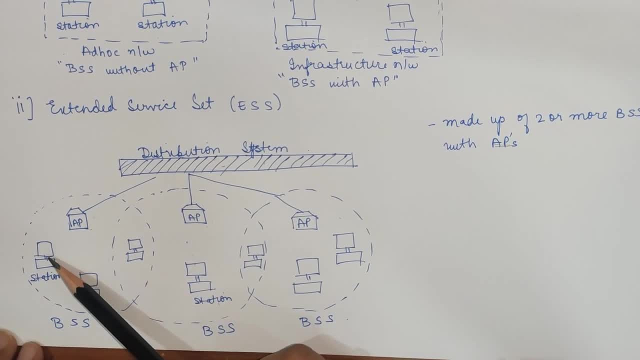 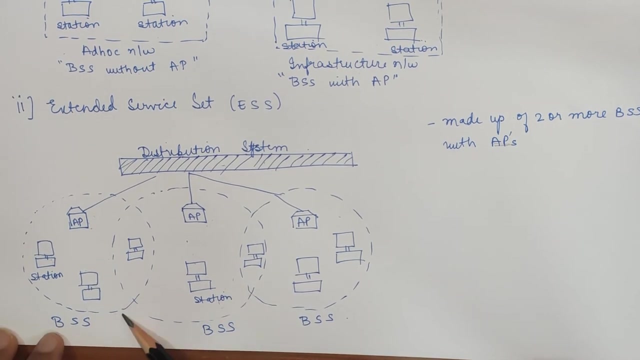 This is the way how they communicate, means if we want to communicate- like, for example, this station want to communicate with this station, they can directly communicate with the help of access point. But what happened if station? if this station wants to communicate with this station means both are of different, different BSS. they can communicate only via and distribution distribution system.